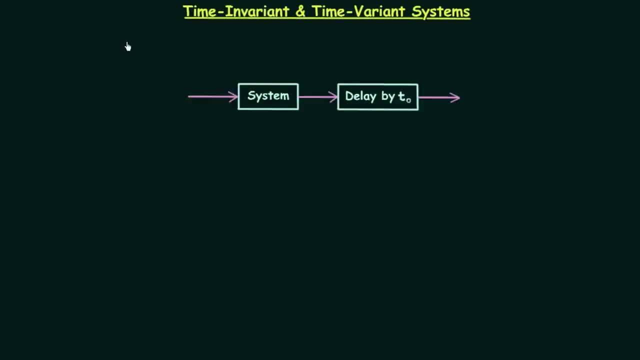 Till now we have completed static and dynamic systems, causal and non-causal systems, and the next classification is time invariant and time variant systems. So in this presentation we are going to discuss what are time invariant and time variant systems. We will also solve two examples to understand the topic in much better way. This particular property of systems. 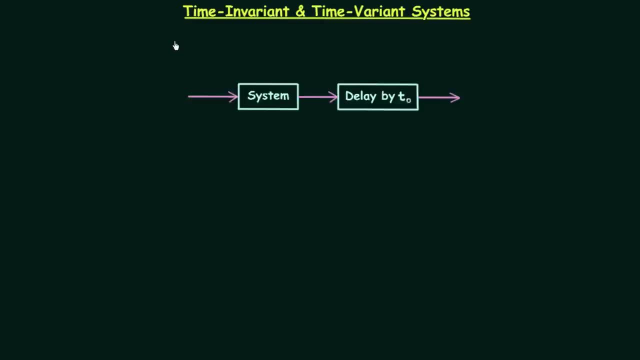 is very important. Time invariant and time variant property is important because we will also use it in LTI systems, linear time invariant systems. So let's start the discussion and, like usual notation we are using till now, x will be the input. x will be the input. 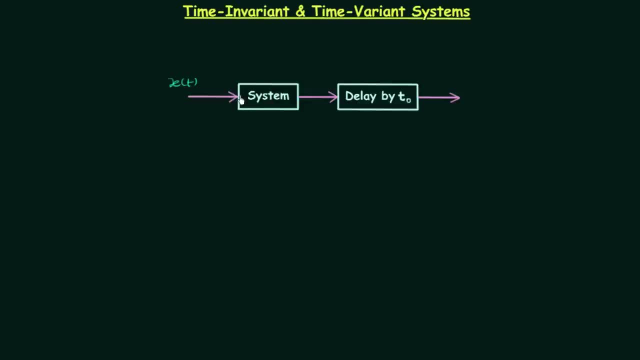 to the system. This is our system and we need to check if this system is time invariant or not. And this system will give us output y. but there is one change: Instead of directly recognizing this output y, we will first provide a delay by t0. So we have another. 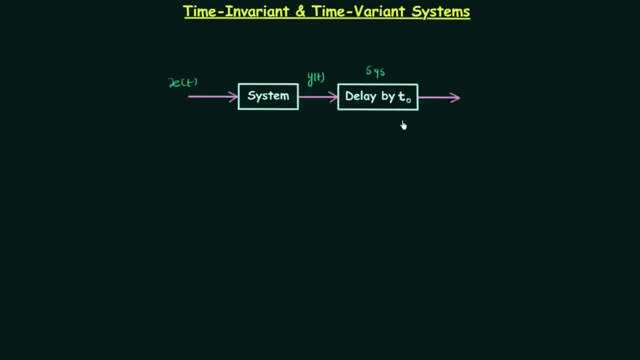 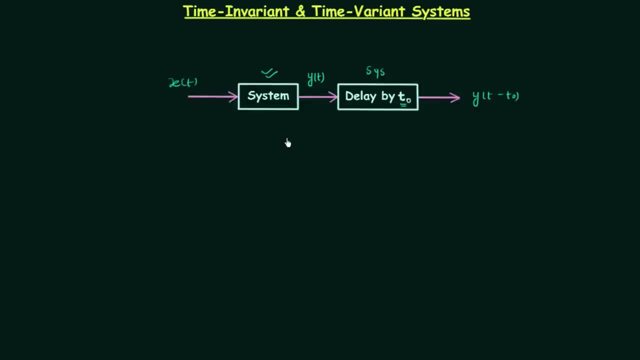 the same thing. So let's start the discussion and, like usual notation we are going to do, I want to provide the delay to the input itself and then I will pass it through the system and I will see if the two outputs are same or not. 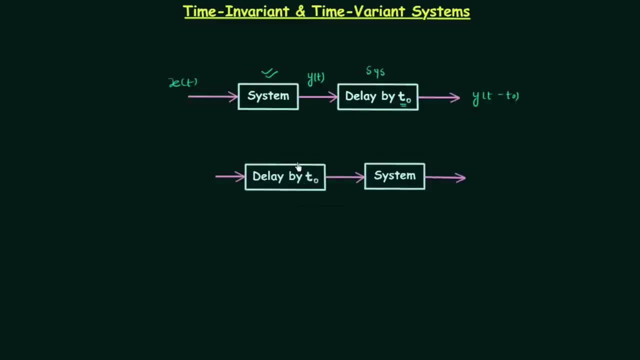 So let's see how we can do it. You can see here: the first system is the system providing the delay of t0 and the second system is the system under analysis. So what I will do, I will provide the same input x to the system providing the delay. 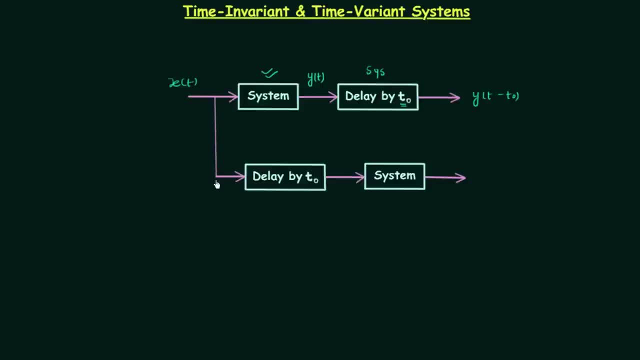 So we have the connection like this: the same input, xt, is given to the system providing the delay. So the first output we will get will be xt-t0, xt-t0.. The input was xt and we have provided the delay by t0.. 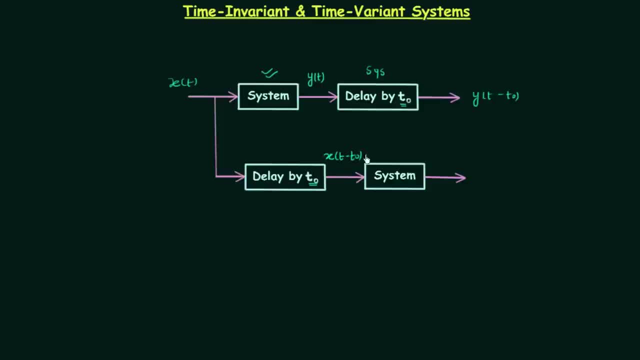 So we have xt-t0 and now we will feed this xt-t0 to the original system and we will have a output. let's say y-t. Now there are two possibilities. In the first possibility, y-t may be equal to y-t0 and in the second possibility it may. 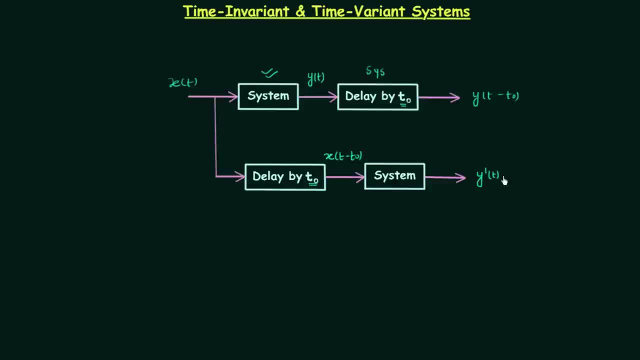 not be equal to y-t0.. So let's analyze the two situations. In the first situation it is equal to y-t0 and in the second situation it is not equal to y-t0.. And when it is equal to y-t0.. 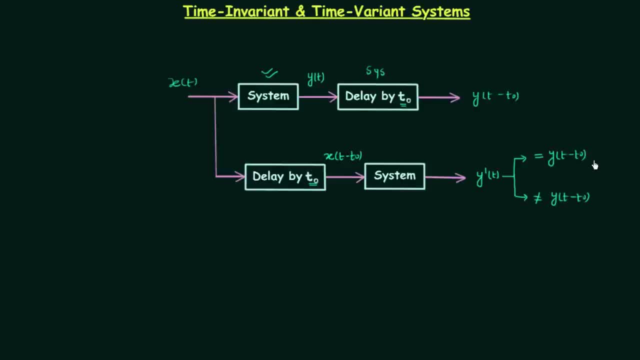 When it is equal to y-t0, we call the system as time invariant system, time invariant system, and when it is not equal to y-t0, we call it time variant system. So I hope you now understand what is the difference between time invariant and time variant system. 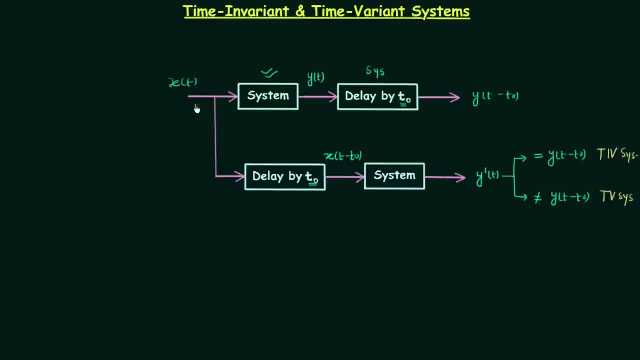 Let us understand the summary of this discussion. We have input xt, and we have one system whose time variancy We want to check, and when xt is provided to the system, the output produces yt. This is what we have Now to check. if the system is time invariant or time variant simply provide the delay of 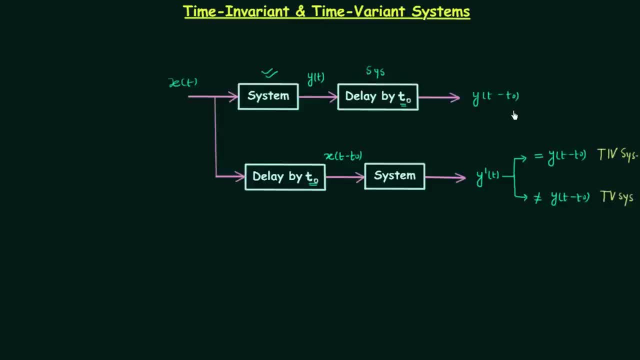 t0 to the output of the system. You will have yt-t0.. In the next step, directly provide the delay to the input itself. You will have xt-t0, and then feed it to the system. You will have y' or y'-t. 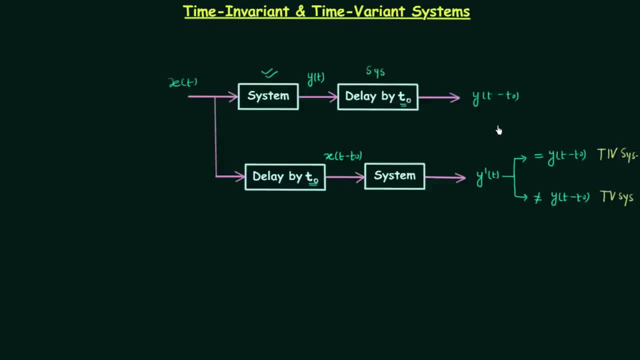 And if the output is yt-t0. Then you will have xt-t0.. The output in the second case is same as the output in the first case. The system is time invariant system, And if they are not same, the system is time variant system. 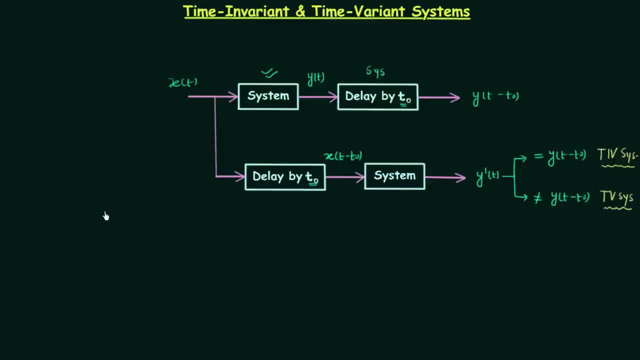 If you want to write down the definition, you can write down. a time invariant system is a system in which any delay provided in input must be reflected in the output. This is the definition, and we have already understood how to check if the system is time invariant or time variant. 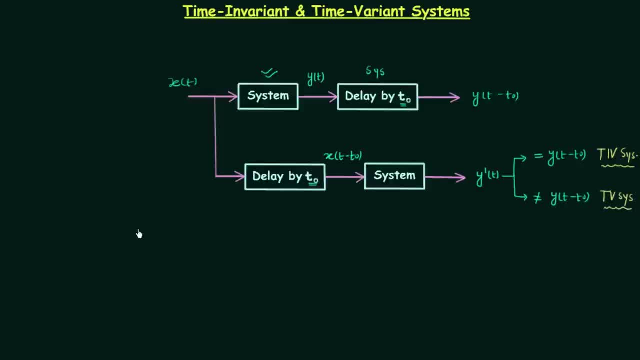 And this will be same process you have to repeat while solving the problems. Now it's time to solve the first example in this lecture, And in this example, output yt is equal to x2t. This means xt is the input of the system and this system is giving us the output which. 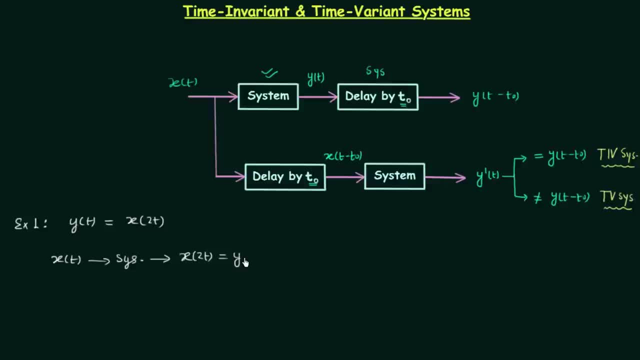 is equal to x2t, So x2t is yt And we need to find the output. We have to find the output, We have to find the input out if this system here is time invariant or time variant. so let's see. 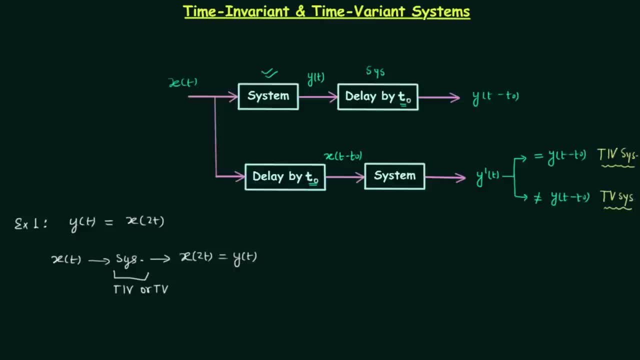 how we can do it. the process is very simple. we have already seen how to find out if the system is time invariant or time variant. so in step number one, in step number one, simply provide the delay to the output. output is yt and we will provide the delay by t naught and we will have yt minus t naught and yt is. 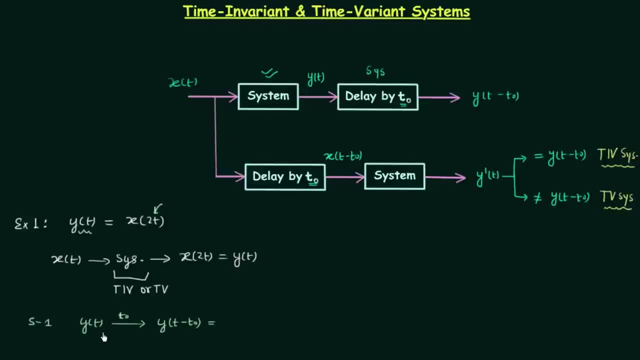 equal to x2t. so simply replace this t by t minus t naught, so we will have x2t minus t naught. simplifying this, you will have x2t minus 2t naught. this is step number one. in step number two, instead of providing the delay to the output, we will provide the delay to. 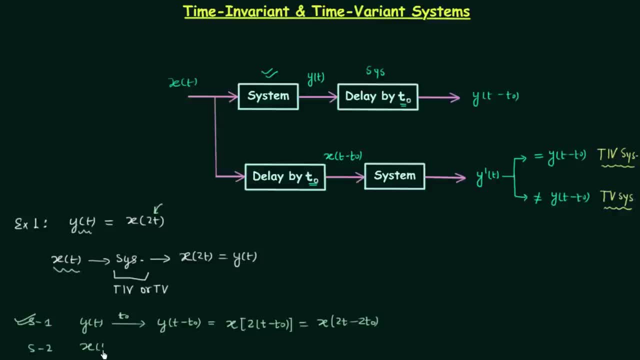 the input. the input is x t, so let's provide the delay of t naught, the same delay as the step number one, and this will give us x t minus t naught. now we will feed this as the input to the system, our system, here. so this will be. 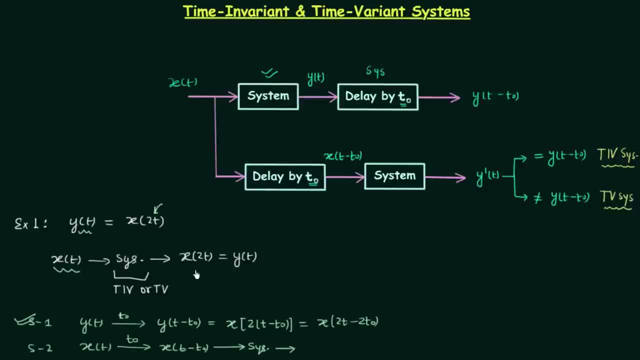 given to the system and the system is having the tendency a to perform the time scaling. this is time scaling operation. it is multiplying 2 to the time. so what will you write down the output? now there are chances of mistake. you may write down the output by simply multiplying. 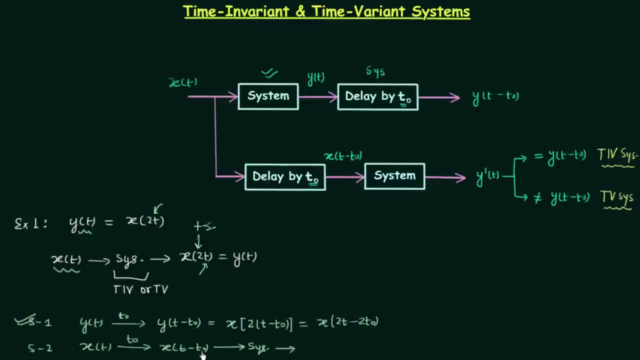 2 to t minus t0. but this is not true because it is only performing the time, scaling on the time itself, not any constant. this t0 here is the constant. it is not varying. so we will have x inside the bracket. 2t minus t0. don't multiply this 2. 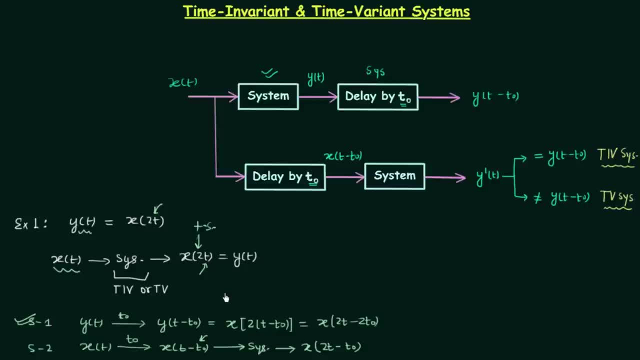 to this t0 also because system is performing the time scaling, and time scaling is only performed on the independent variable, which is t in this case. so this is what we have in step number two. now compare this and this, compare the output in the first case and output in the second case. you will find they are not. 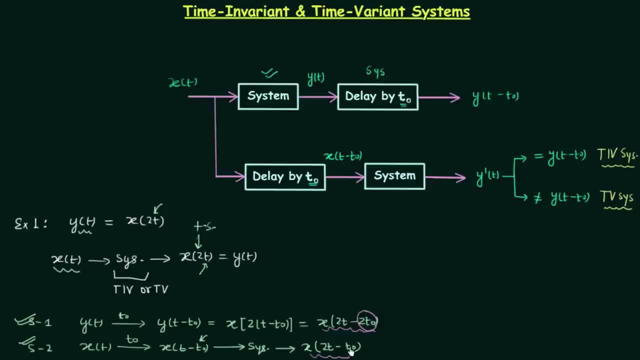 same. here we have 2 t0 and here we only have t0, so the system will be time variant system. so this is the process to check if the system is time invariant or variant. now let's solve the example number two. in this example, output yt is equal. 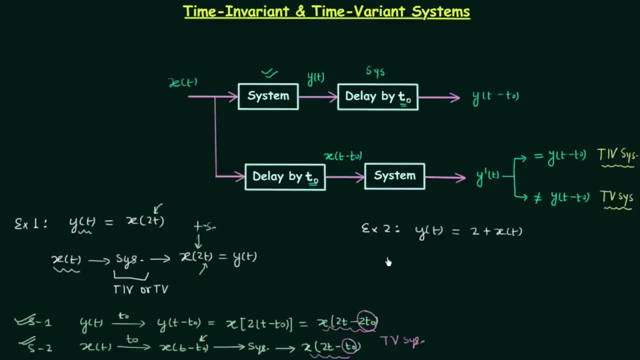 to 2 plus xt. again, you can assume how the system is working. you are providing Xt to the system and the system is giving us the output, which is 2 plus xt. this is the output yt, and we need to find out if the system is time invariant or time variant. 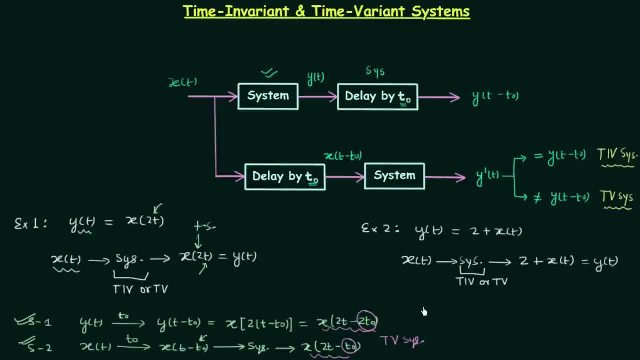 we will follow the same process in step number one. in step number one, we will provide the delay to the output yt and this will give us 2 plus X, T minus T naught. instead of this T, we will have T minus T naught. this is the output in this step number one. in step number two: 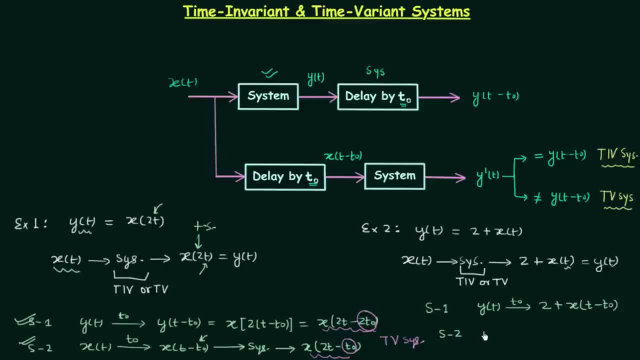 we will provide the delay to the input itself. so, providing the delay, we will have X T minus T naught. this is after providing the delay, and now we will feed this to our system and the system will give us the output, which is 2 plus X T. 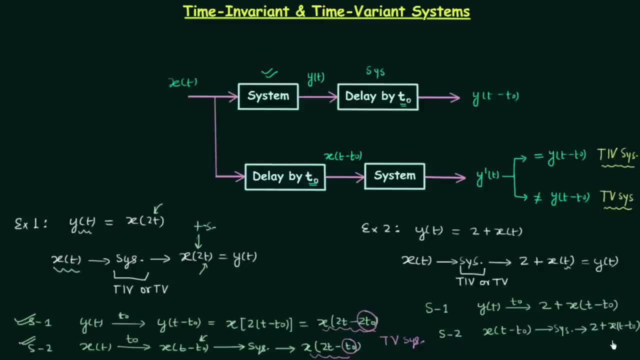 minus T naught okay, and if you see the two outputs you will find they are same. so this time the system is time invariant system, time invariant system. so there is one conclusion which you can derive from these two examples. the conclusion is: whenever the system is time invariant, 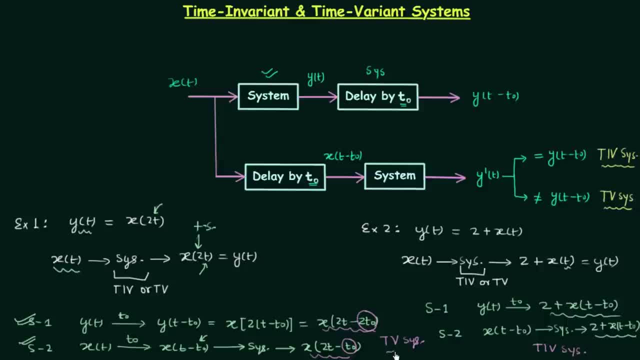 system is performing the time scaling, it is going to be time variant system. and when the system is performing the amplitude shifting- this is the case of amplitude shifting- the system is time invariant system. so this was all for this lecture. in the coming presentations we will derive few more important. 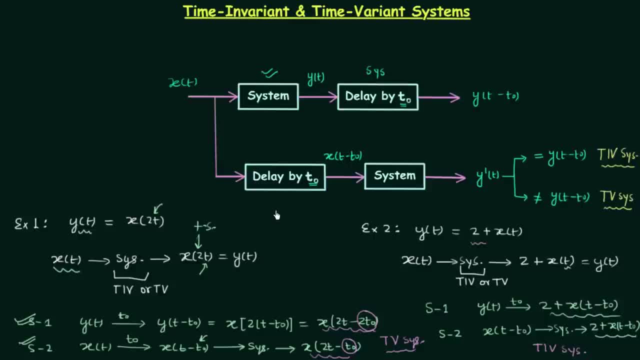 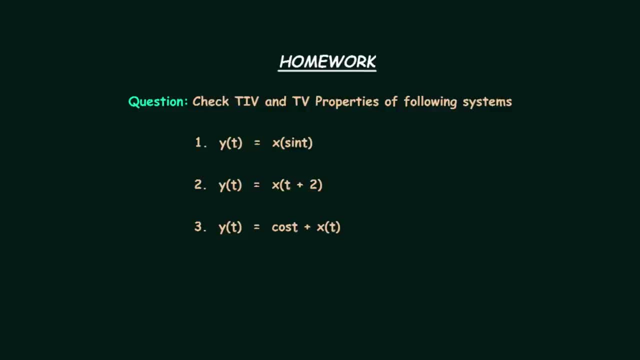 results based on time invariant and time variant systems. in the coming presentations we will derive few more important results based on time invariant and time variant systems.